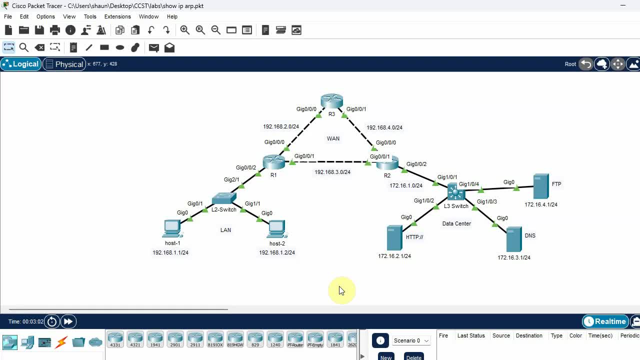 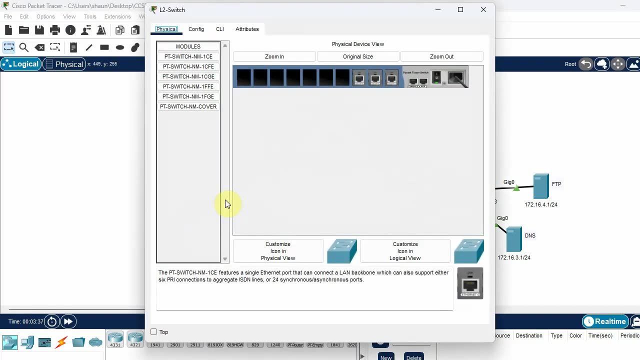 that's triggered by that network traffic, to start populating the ARP table with the MAC address needed for setting up that communication between source and destination. What I'll do is I'll show you the ARP tables currently as they exist, without any network traffic. So I'll go to layer. 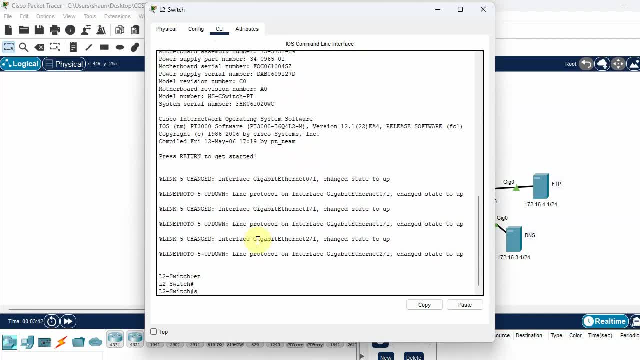 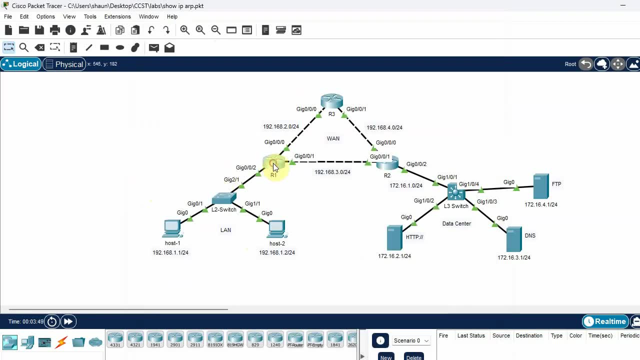 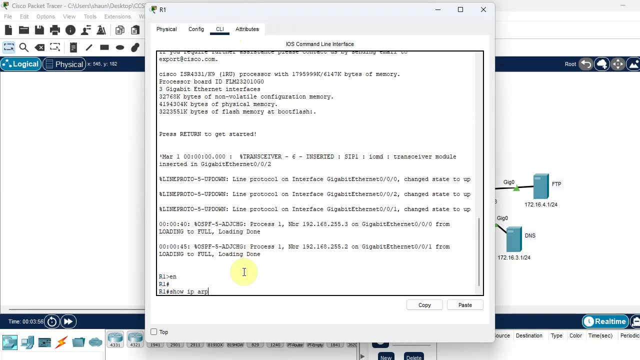 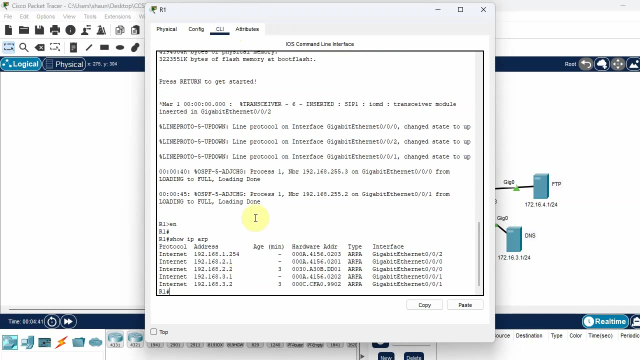 two switch and I'll just show you that layer two switches don't have an ARP table. Nothing there. I'll go to R1 here. use the same command, show IP ARP. You can see that this is populated already, before any traffic has been sent. So you note there's five entries with this. 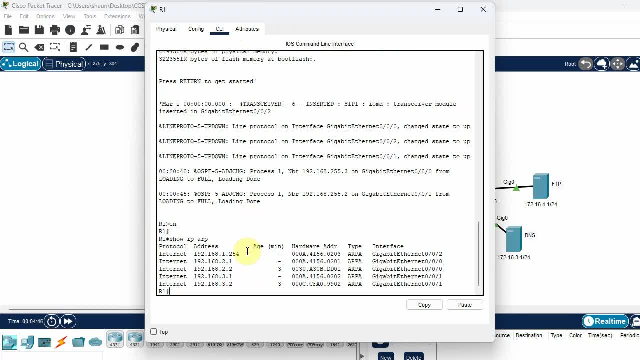 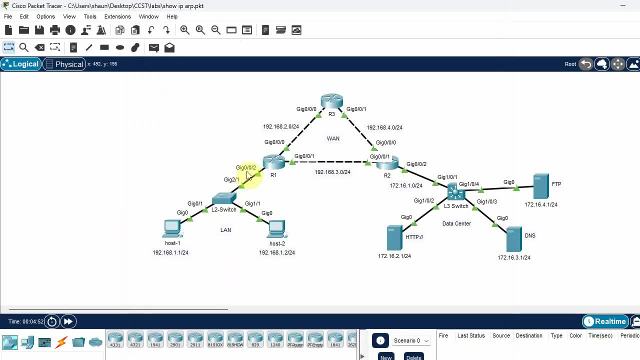 ARP table. Three of them are actually belong to the local interfaces on R1. The 192.168.1.254, that's actually gig zero, zero. Then you've got these other two interfaces: zero, zero, zero and zero, zero one. Now zero, zero, zero is. 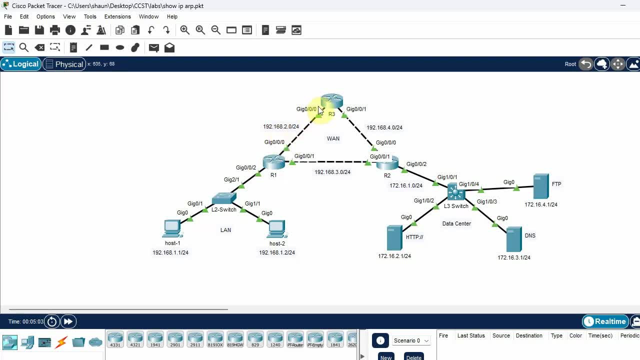 192.168.2.1, and the neighbor on R3, gig zero, zero, zero, that's 2.2.. The same here on gig zero, zero one. this is 192.168.3.1. and on R2, zero zero one, it's 192.168.3.2.. That's what the other two are. 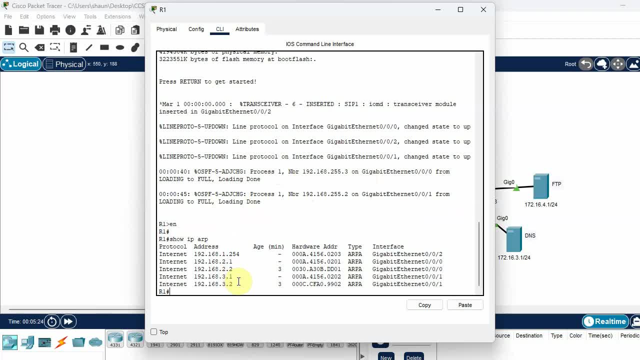 sourced from. So two times two, Two and three. two are actually advertised from a neighbor. There's the age there, three minutes. that's because it's advertised. The other ones are local so they don't have any age on them. 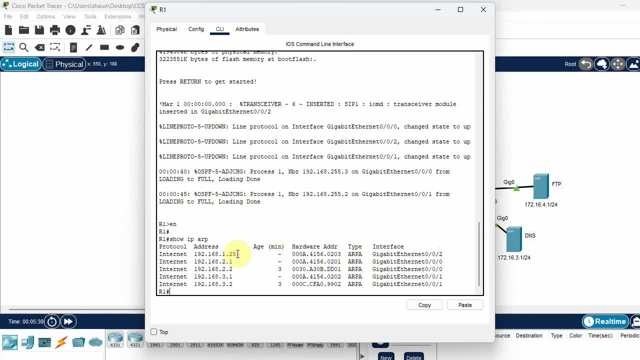 These are the local interfaces where this was learned from. So 192.168.1.254, that's gig zero, zero two, for instance. That's actually a local interface. So the ones that are advertised from R2 and R3, this is zero, zero, zero and zero zero one. That's where it's actually learning it from. 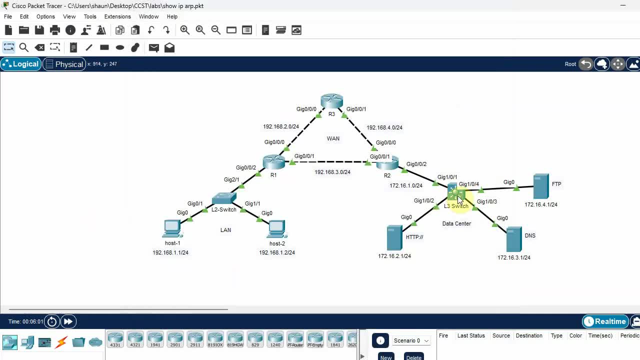 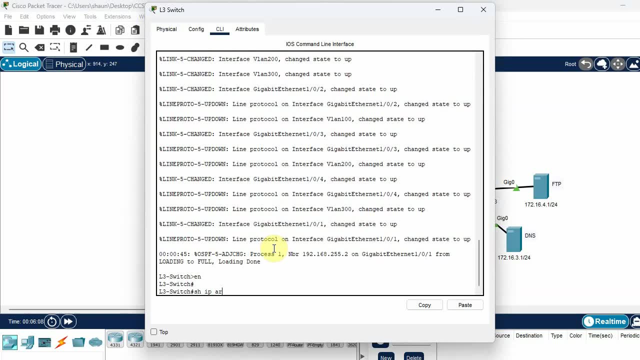 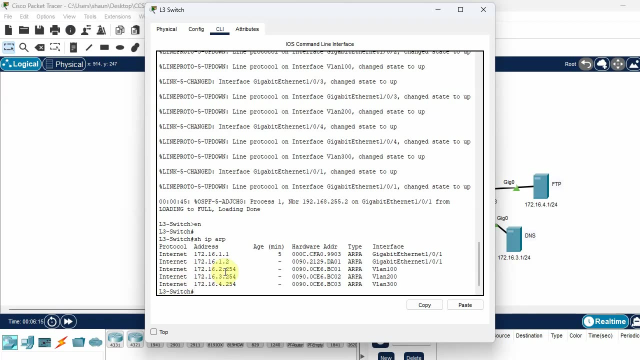 So that's the start of the ARP table. Then I'll go to layer three switch. here I'll do show IP ARP, Since it's a layer three switch. it does have an ARP table. It has the same thing as well. It's got 172.16.2.3.4.254.. These are gateway addresses. 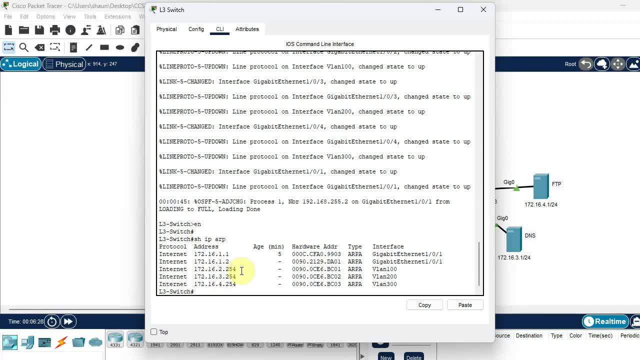 They're called SPIs VLAN interfaces that are configured on the layer three switch. They're actually default gateway interfaces, So they're local interfaces. And the 172.16.1 and 2, the 1.2 is local because it's got no age- And the 1.1, 172.16.1.1,. 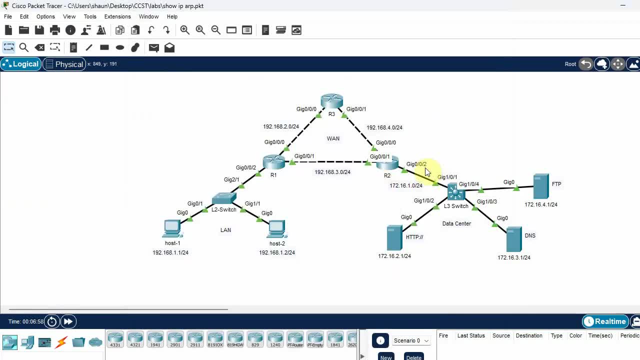 this is the R2 that's advertised. That's the IP address of gig zero zero two on R2.. Now what I'm going to do is I'm going to start a ping from host 1 to 172.16.2.1 to generate some traffic. 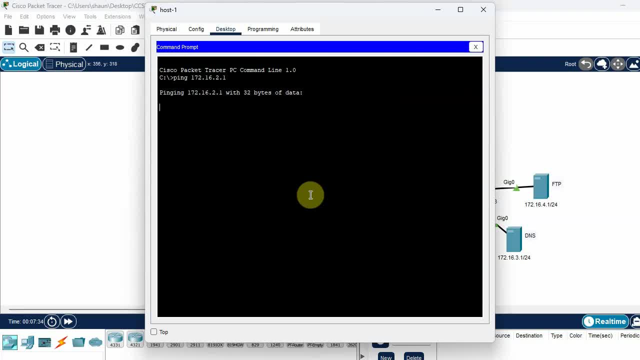 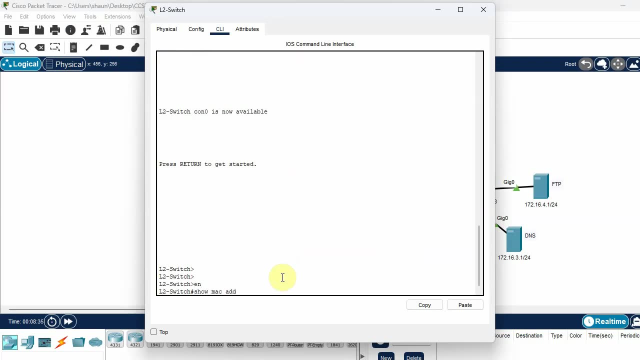 So that works okay. Now I'll look at the MAC address table on the layer two switch. You can see there there's gig zero one. It's in there because that's where I sent the ping from. I'll show you IPR and there's no ARP information here. just to show you. 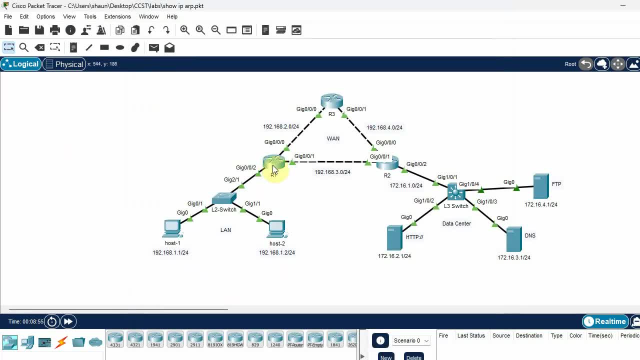 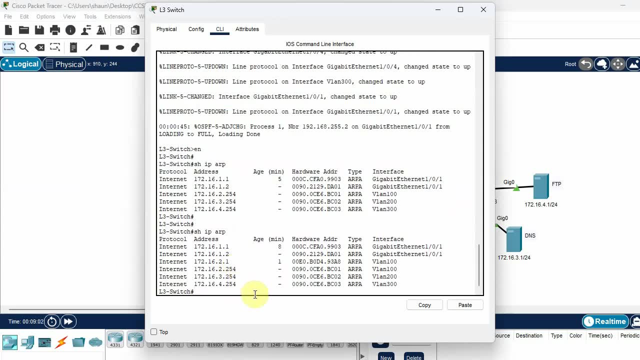 that you anything? because they don't support ARP tables And I'll go to layer three. switch here. show IPR. So the only new one I've got there is this: 2.1.. That's VLAN100.. That is the HTTP server. So it's got the mac address of the HTTP server there. 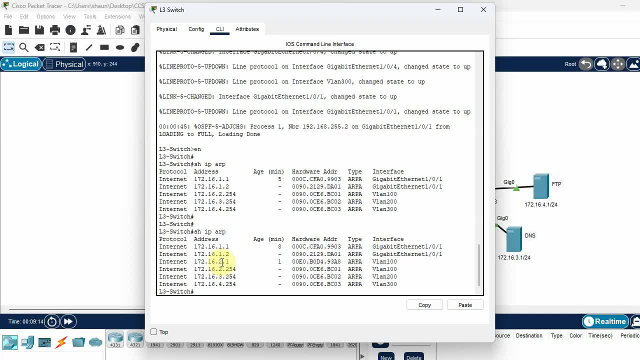 So it's got the MAC address of the HTTP server there, That's VLAN100.. That is the HTTP server. So it's got the MAC adress of the HTTP server there and also the 192.67.225.8.1 there. 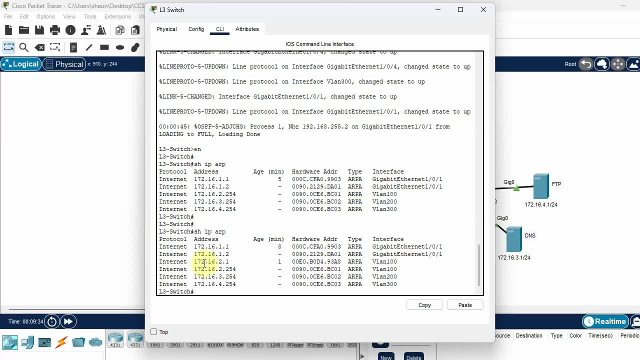 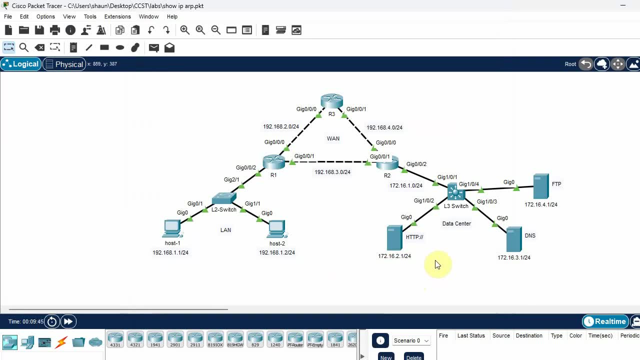 and also the VLAN assignment, VLAN 100.. So what happened is Host1 sent a ping to the HTTP server and what happens is the HTTP server returns its MAC address to the Layer 3 switch. So now it's actually in the Layer 3 switch. 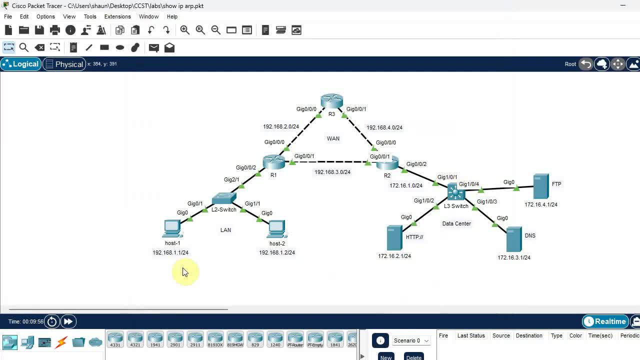 It doesn't go any further than that, but it's there so that when the actual ping arrives, the Layer 3 switch will know how to do the addressing. So two things happen then. First thing is that the web server responds with its MAC address. 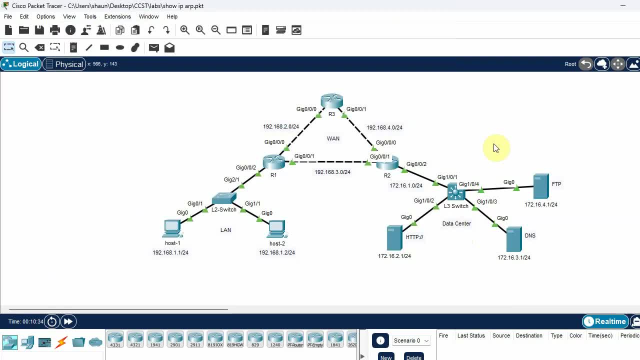 So what happens is in the Layer 3 switch that gets installed into the MAC address table, There's also an ARP table entry as well that associates the IP address with the MAC address and that's used for addressing as well, Since all Layer 3 devices, whether it's a router or a Layer 3 switch- 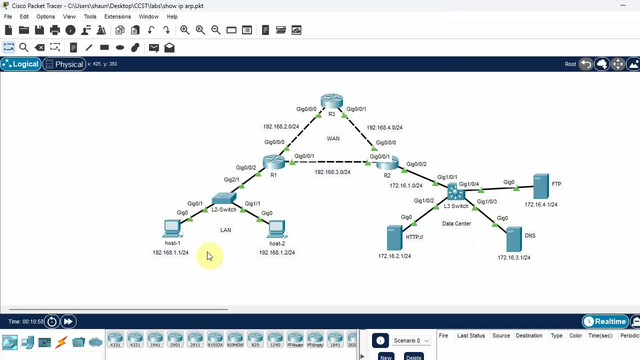 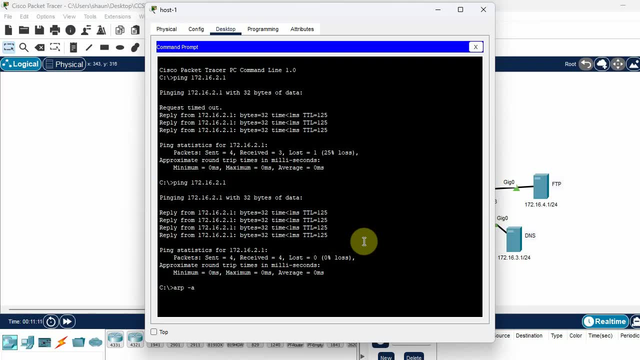 will do. the addressing both MAC address and IP address Go to Host1 as well. The thing that ARP does is it creates an ARP tree and the host for the host. So ARP slash A. So you notice here it's got the MAC address of the default gateway. 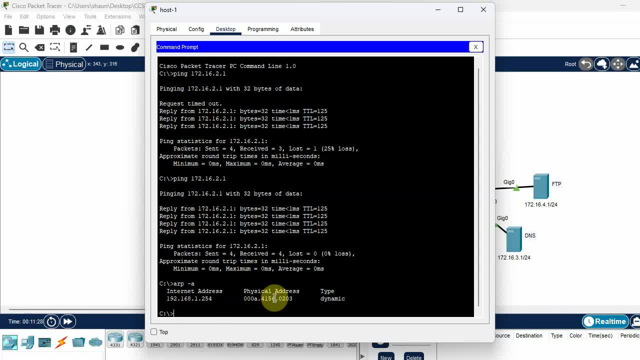 So this is the other part that ARP does. It finds the MAC address of the default gateway so it can actually start addressing. So this MAC address becomes the destination MAC address for all traffic outside the local subnet. It goes right to the default gateway. 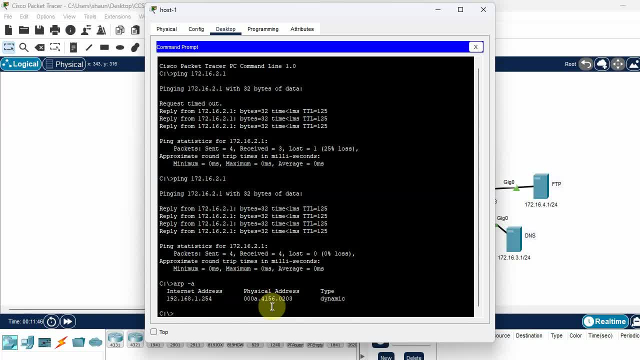 That's R1. Then R1 will do the routing and send it off to the remote location, to the remote subnet. So there it is, ARP 192.. Once again ARP 192.. 168.1.254.. And there's the destination MAC address. 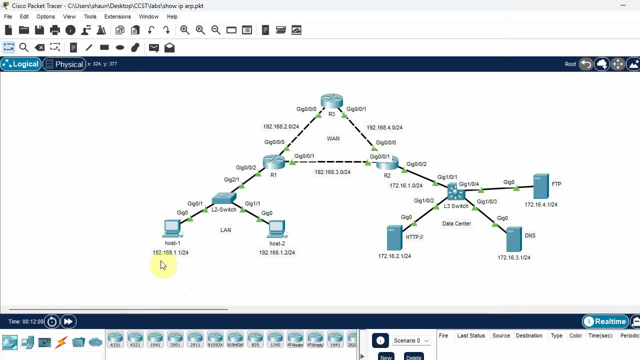 When the pack is leaving Host1, the source IP address would be 192.168.1.1.. The destination IP address would be 172.16.2.1.. And that doesn't change per hop between source and destination. It's only the MAC address that changes as it hops between different Layer 3 devices.